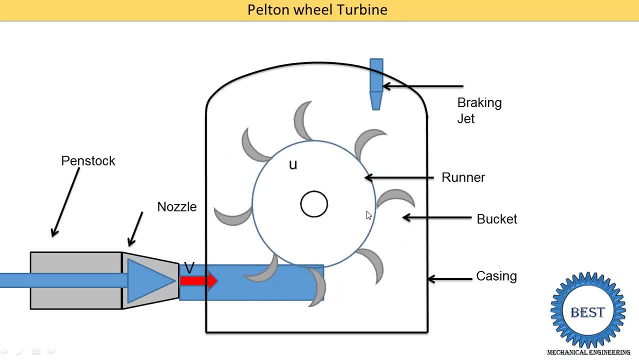 u, that's at the workings of a bucket. after this is a bucket, this is the runner on the runner, the bucket is installed. another part is the casing. before that, i request to subscribe my channels, like my video and comment on the video. this part is known as the casing. this is the vibrating part. it is outer parts. we learn why the casing is. 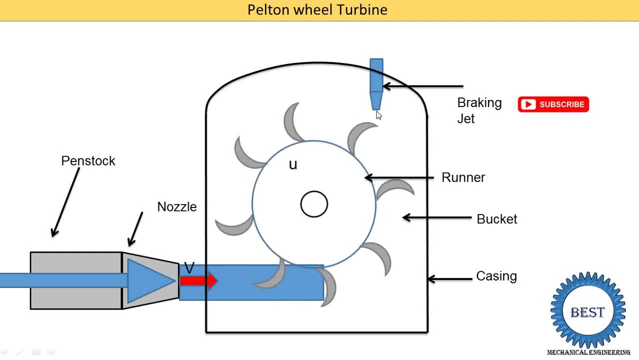 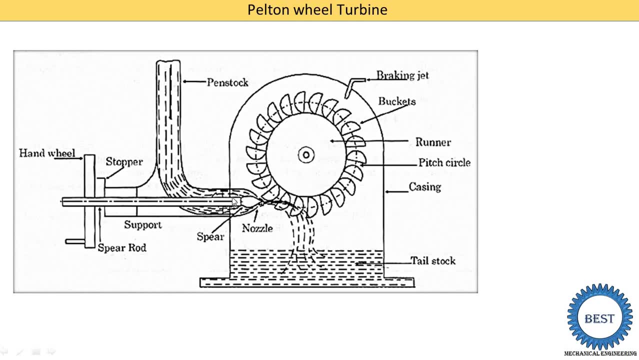 provided this part is the breaking jet. okay, so this is the breaking jet of the our pelton wheel turbine now in exam. it is asked then you draw like this figure or a last one. so this is the last. one figure is the simplest to draw so it is a little bit complicated. the both is correct if 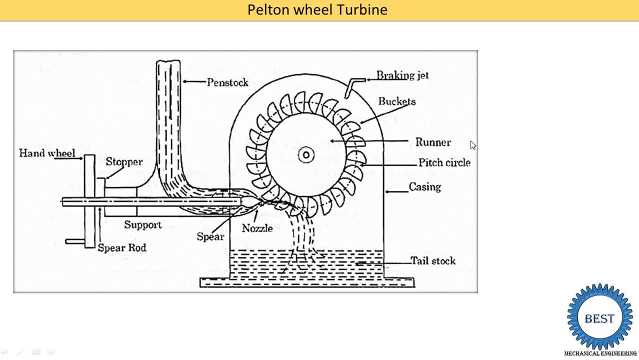 you draw in the examinations. so these are all the component. now we learn the introduction, so first you need to writing down the only six point that i teach you right now. so first is write down. the paladin is a impulse turbine. impulse turbine means in a turbine, the water supplied, which have only 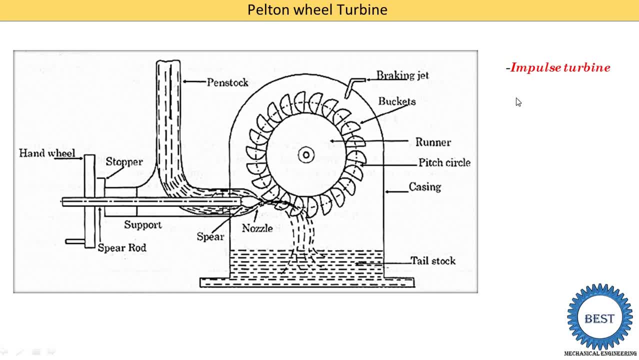 kinetic energy. they have no any pressure energy. it's known as the impulse turbine. second is that the flow of the water is the tangential flow. tangential means the water coming from the nozzle is strike to the turbine blade. it's touch only the one part of this runner, that is known as the one. 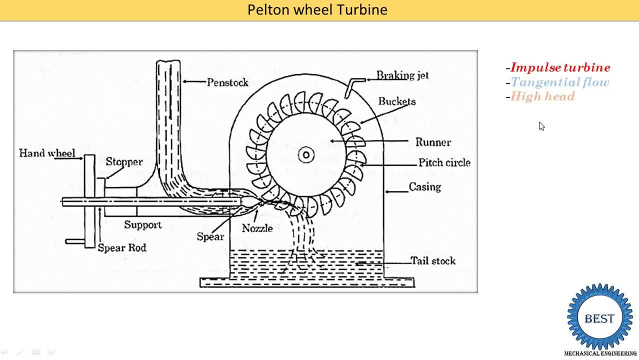 point. it is known as the tangential flow. next one is the high head means. pelton wheel turbine is used in a such a dam which have a head is greater than 300 meter. it is known as the hydra high head turbine. next is the pelton. 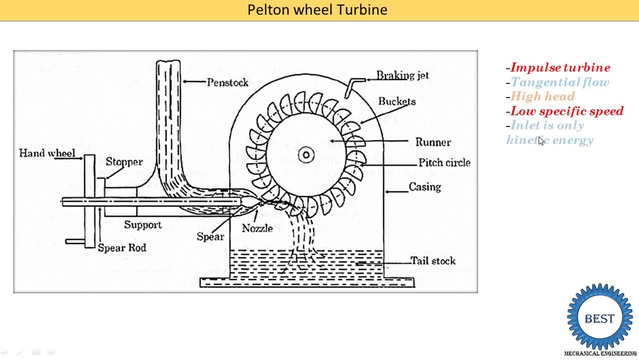 wheel turbine have a low specific sphere. next point is: inlet is only kinetic energy. as we already study in impulse turbine, the inlet is only kinetic energy and pressure at the inlet and outlet of the turbine is atmospheric. so this is the inlet part of the turbine. it is atmospheric. 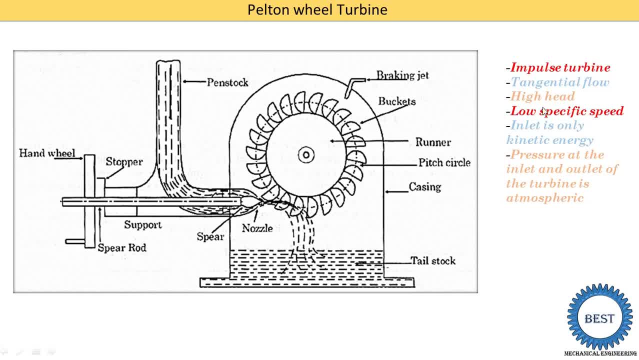 outlet. so in the whole turbine the pressure is remain constant because, as the inlet it is impulse, turbine and inlet have only kinetic energy, so there is a no change in this pressure. okay, so when this question is asked in the exam, you draw this, draw just these figures and writing. 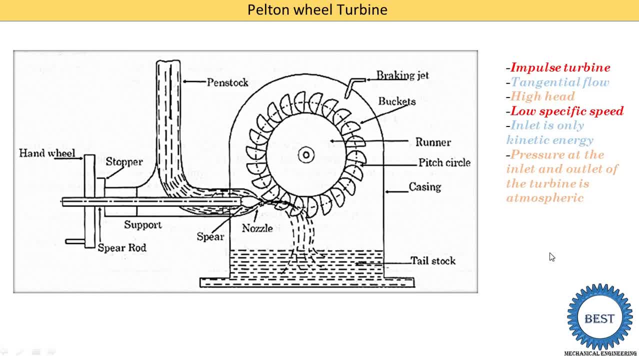 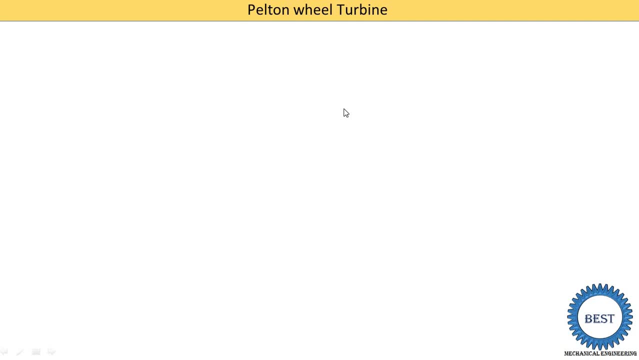 down the six point and it is easy to examiners to mark you now the high head. then another point is added, that is, a low quantity of water is supplied when the head is high, then it's supplied as a low quantity. so these are the different six points. now we understand it's. 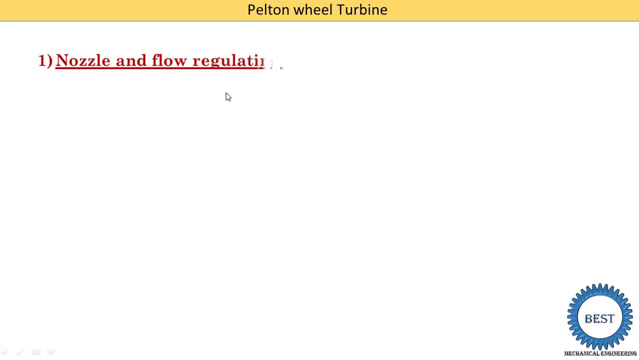 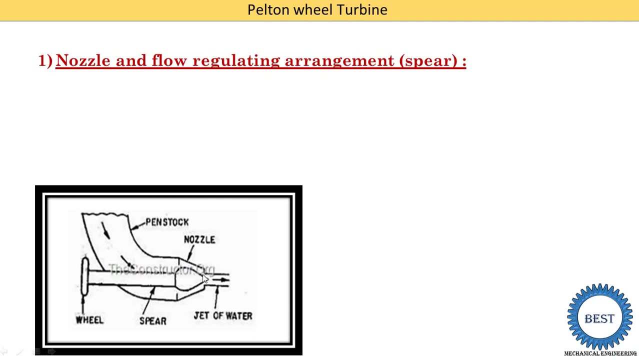 different component. the first one is the nozzles and flow regulating device that is known as the spheres. so first, this is the figure, this is the nozzles, and inside of these penstock and the nozzle there is a one sphere is provided. okay, so nozzle. so first we understand nozzle, nozzle. 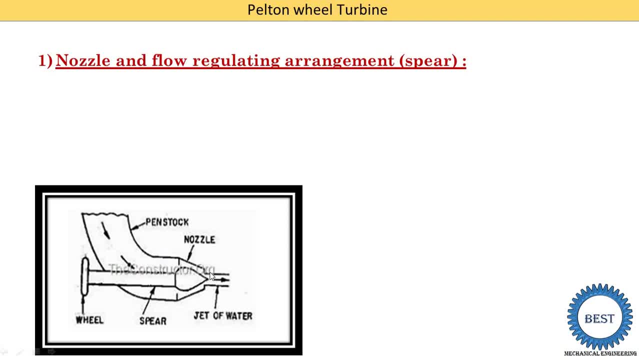 have a conical shape. it is generally used to convert the pressure energy into the pressure kinetic energy. so, whatever the pressure energy in a water in the penstock is converted into kinetic energy at the outlet of the nozzles and it's strike on a turbine plates. okay, so nozzle. 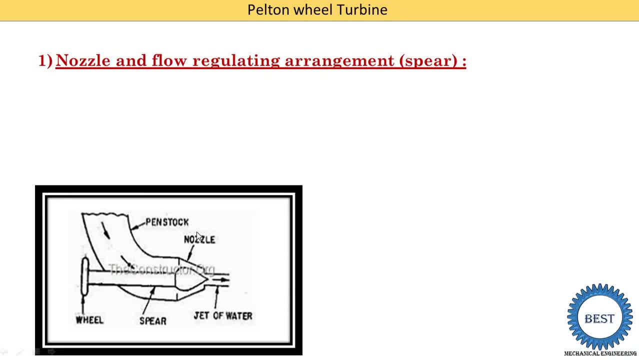 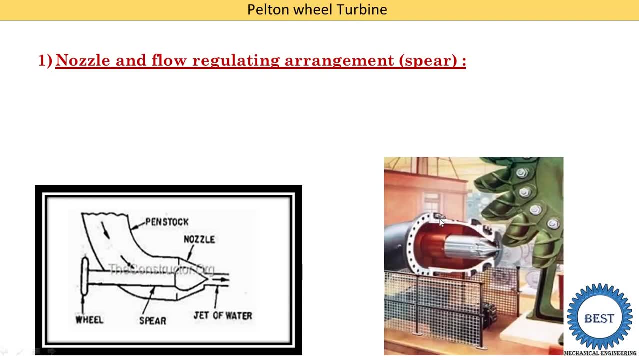 have conical shape. it's used to convert kinetic energy- sorry, pressure energy- into kinetic energy. now why this sphere is used. so first we i show you another image, that is, a sectional view of this nozzle and sphere. this part is known as the nozzles. inside this nozzle there is a sphere that 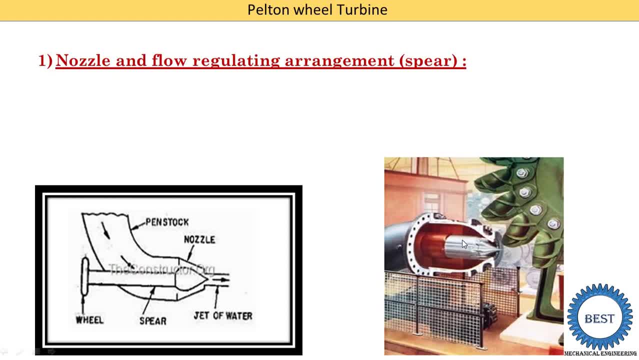 is a bucket of this turbine. the sphere have a also conical shape and this sphere is used to control the flow rate of the water. sphere is used to control the flow rate of the water and this sphere is controls by manually, by rotating this wheel, or this wheel is also operate by automatically. 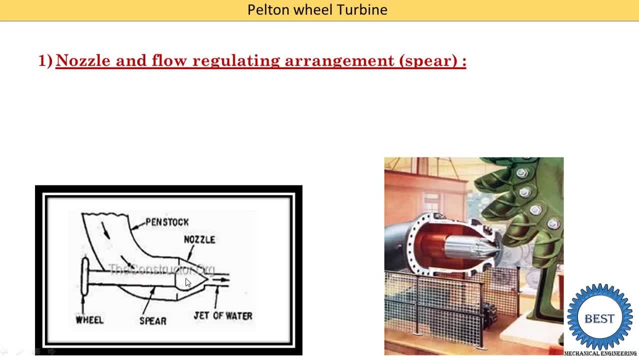 so this wheel or a sphere is moving in two direction, that is, either moving inside the or removing from the outside the nozzles. okay, so when we supplying this sphere inside the nozzles, the nozzle area is reduced and water supply is reduced. when we push this sphere outward direction, okay, then the nozzle area is increase. 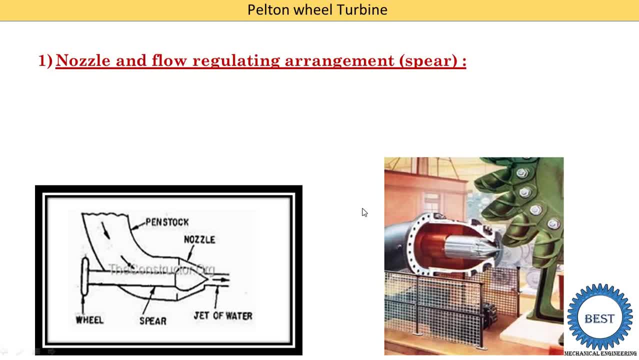 and water supply is increase. okay, so quantity of the water is required change due to the governing mechanisms and maintaining the constant speed of the turbine when we require to run the constant speed, so we need to change the quantity. that we learn later on the governing mechanisms. okay, so these are. 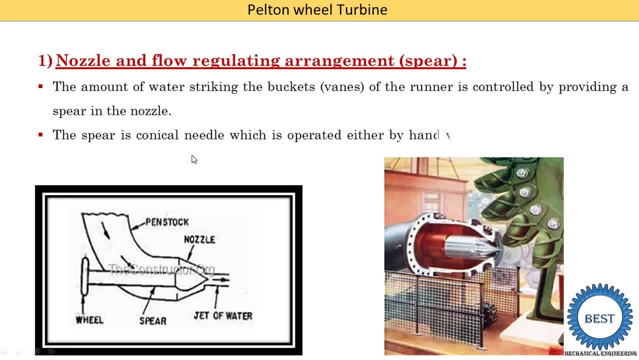 the working of the nozzles and sphere mechanisms. so sphere is conical needlework which is operated either by hand wheels and automatically and it is used to controlling the flow rate. again, I revise that it's know either inside or outside. when this sphere is moving inside, the area of the nozzle is reduced. 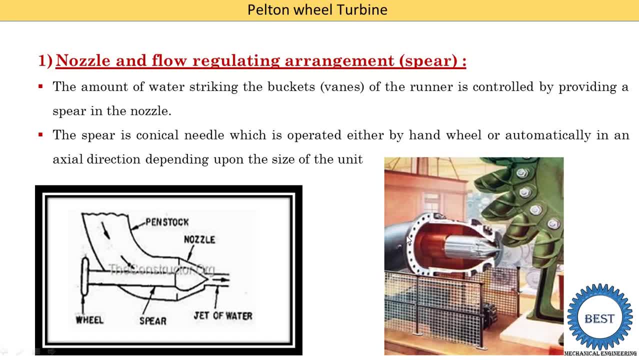 quantity of the water is reduced. when we pull outward directions then the area of the nozzle is increased and both were controlled. that will help creamy movement to the and water supply is increased. when water supply is increased, the turbine speed is increased. when water supply is reduced, turbine speed is reduced. so this is the working of nozzle. 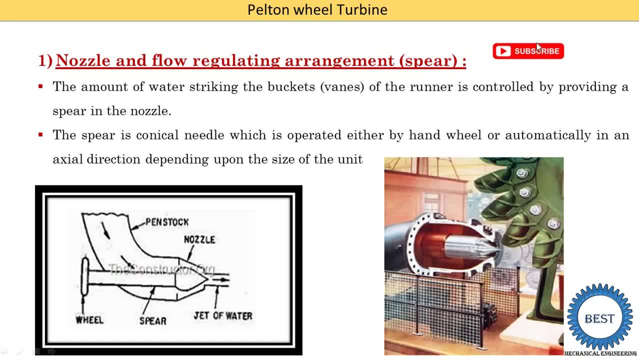 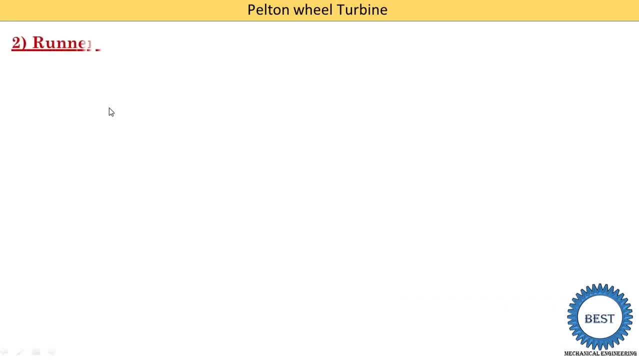 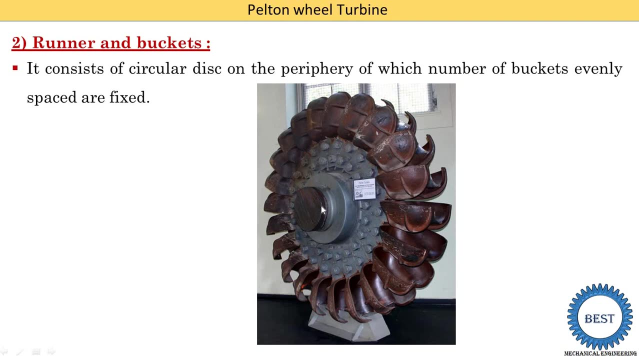 and spheres. if you learn something, then subscribe my channel, share with your friends and comment on the video and like. like and comment give us the motivations to make the more video now. second, we understand the runner and bucket, so i explain this by using this one figures. runner means it is a one circular dicks and this runner is mounted on a shaft, so this 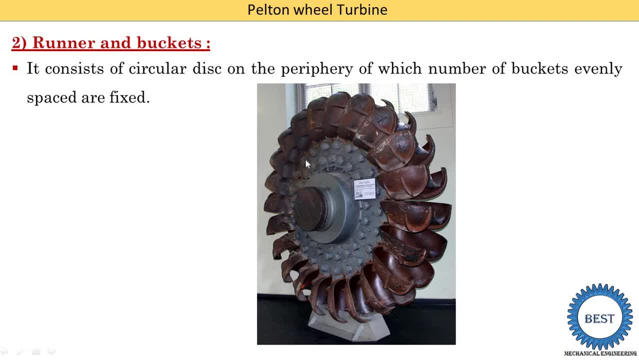 the part is the shaft. on the shaft, this silver color portion is our runner. ok, so runner is a circular dicks type portions. it is mounted on a shaft. that is only two point. you return on the runner now. another part is the bucket. so on this periphery of the runner, these are 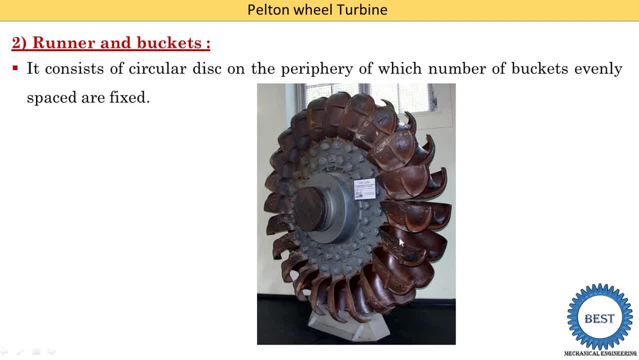 the periphery of the runners. on the periphery of the runners we are mounting a number of the bucket, okay, and it's are mounted on uniform distance on a periphery of the runner. so bucket are mounted on the periphery of the runners on a uniform distance. 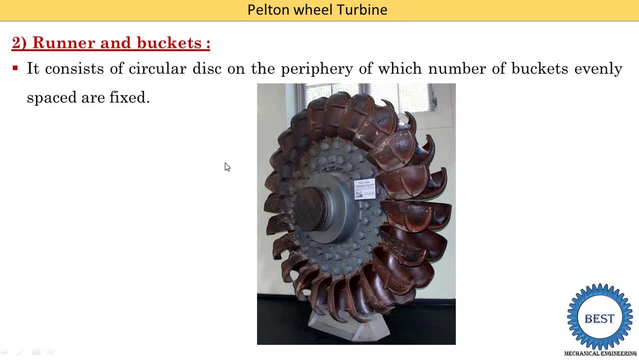 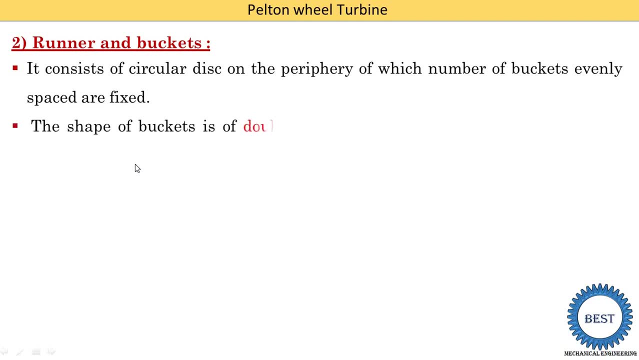 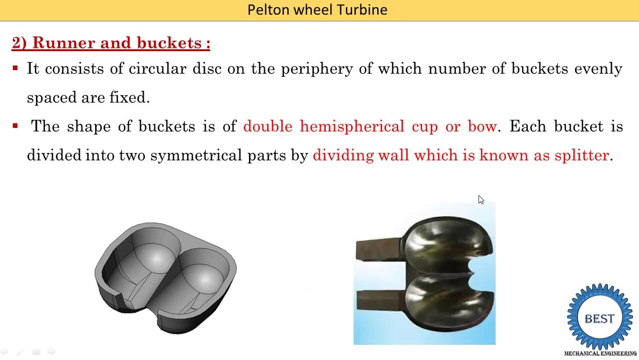 next we learn detail about this bucket, so i removing this figure now. the bucket shape is a double hemispherical shape, so bucket shape is double hemispherical curve or a bowl shape. each bucket is divided into two symmetrical parts. so i show you in this figure so bucket is look like that. so i giving you some simple example. spear means. 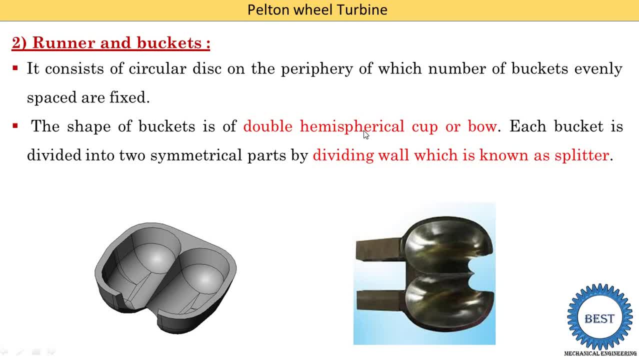 that is like a football or a cricket ball. that is known as a spears. when we cutting this ball or a spear in a two parts, then it is known as the hemispherical. now we cutting the one ball that is divided into hemispherical, now two hemispherical. 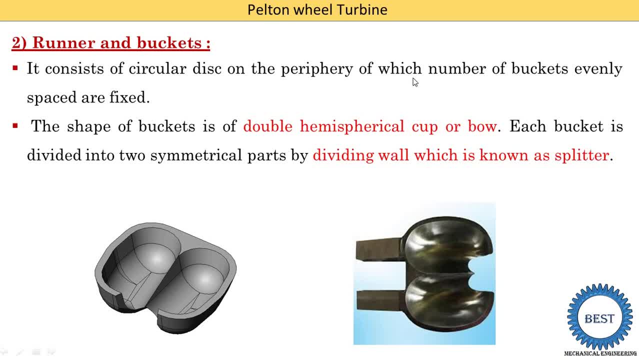 joint, then it is converted into the double hemispherical cup and it's get the shape like this way. okay, when we joining this two hemispherical cup, then we get the double hemisphericals, and this joining part means, like: this periphery is known as the splitter. okay, this part is known as the splitter. 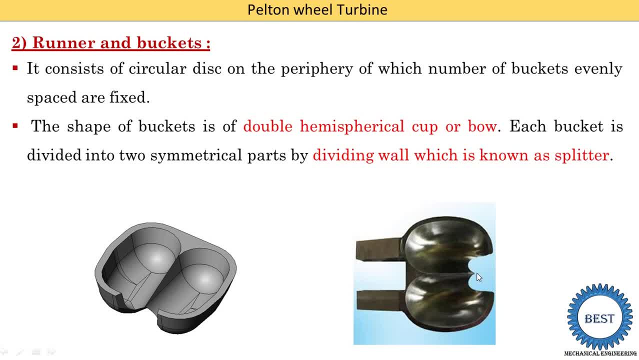 the splitter name itself suggests to divide the water flow in a two parts. splitter means divide the in a two parts. so this splitter is divide the water jet in a two parts. so after striking on the bucket, the water is flowing on from the both the side of the bucket smoothly. 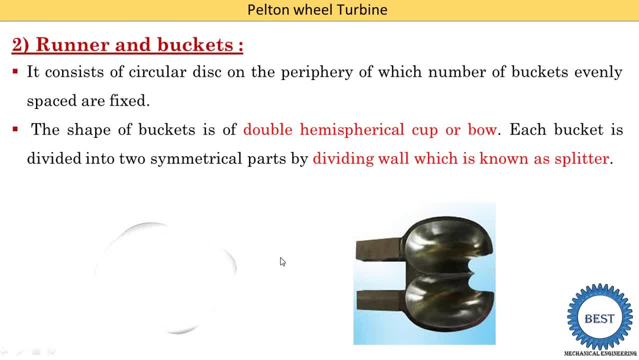 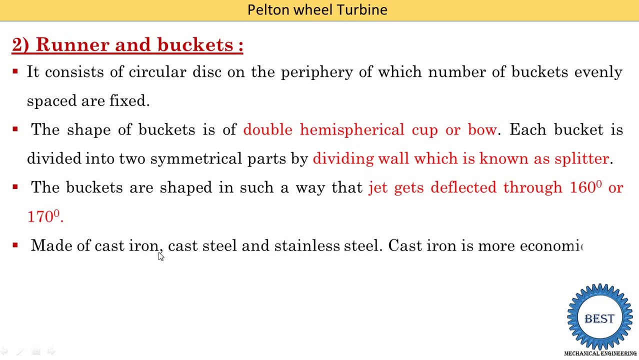 now, another thing is the how number of bucket is requires. what's the dimension of this bucket? so, and what's the angle of this bucket? their bucket are shaped such a way that jet is deflected to 160 to 170 degree. bucket is generally made of the cast iron cast steel. 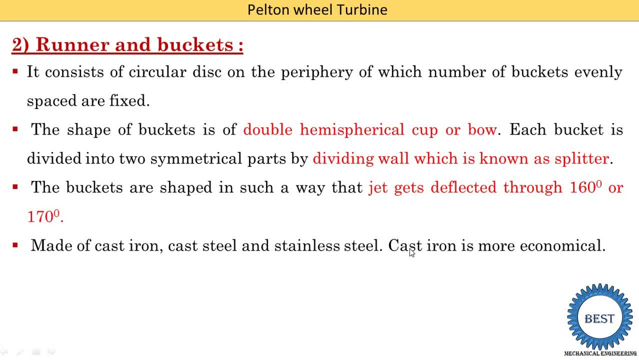 so and what's the angle of this bucket? their bucket are shaped such a way that jet is deflected, and stainless steel- the cast iron, is more economical, but cast iron is the corrosive material so it's react with the metal. so for a long life generally the steel is used either. 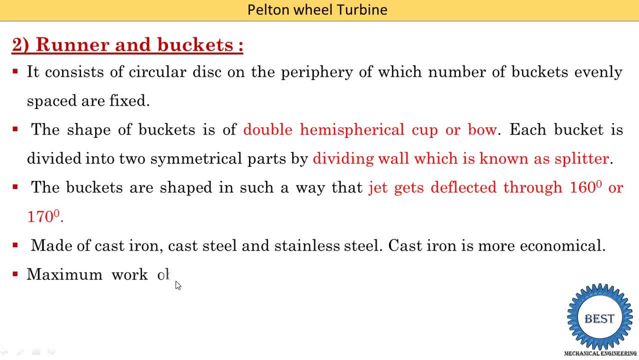 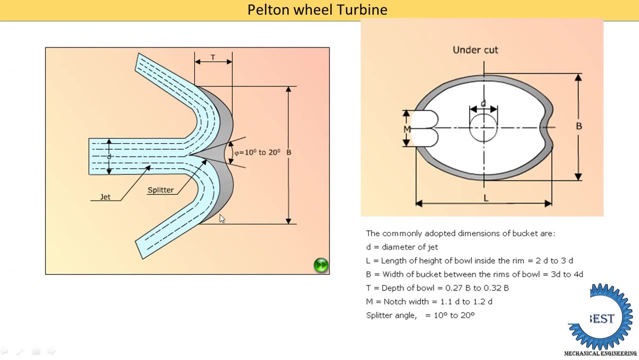 cast steel or a stainless steels. next point is that the maximum work obtained at the 180 degree and typical pelton wheel turbine are 21 buckets. so generally 21 buckets pelton wheel turbine are used. these are the dimensions of the buckets and i covered these topics. 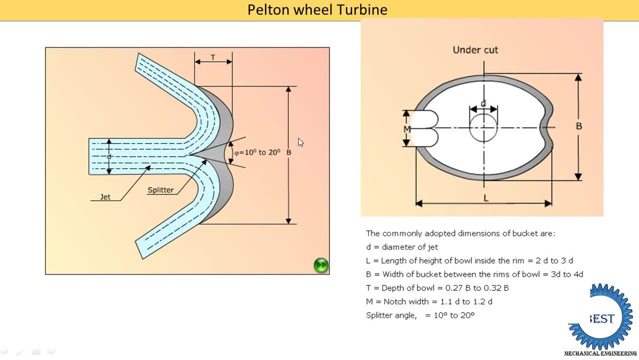 on the design aspect of the pelton wheel turbine later on. now i just focus on the two parts, that is, a length of the bucket and the width. the length and the width are our. the parameters of the of the bucket is specified in the terms of the diameter of jet. this small is indicate the diameter of jet. so length or height of 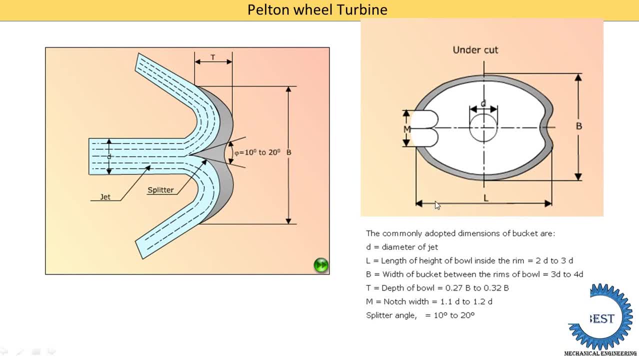 this bowl shape is a two or three times of the diameter of jet. so because diameter of jet is 100 centimeters, then the length is a 200 centimeter or 300 centimeters. another part is the width means. this is the width b, so it is a three to four times of this diameter of a jet. so diameter of a. 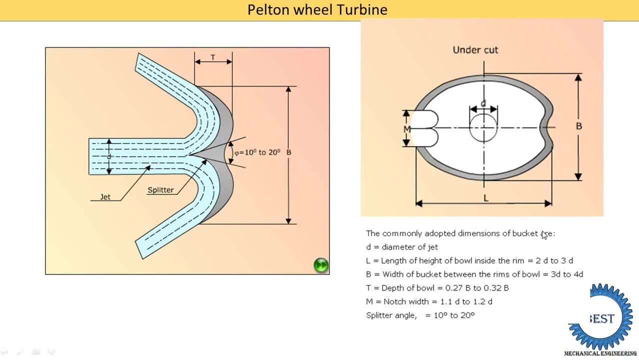 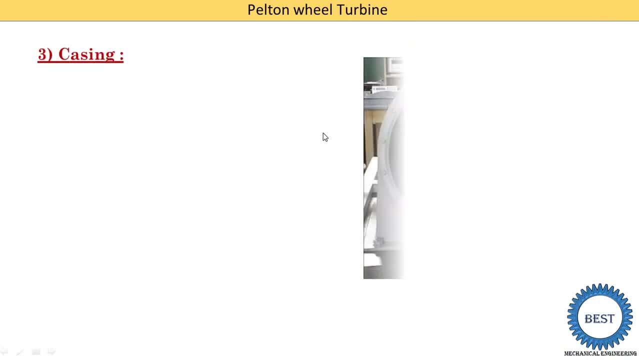 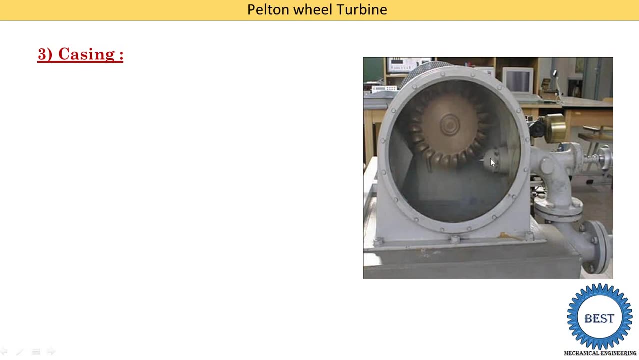 jet is 100 mm, then the width is 300 to 400 mm. okay, so it is directly multiplied. now the next portion is the casing. casing means the outer portions of any device is known as the casing. so this is inside these turbines and this outer part that is a silver color portion. 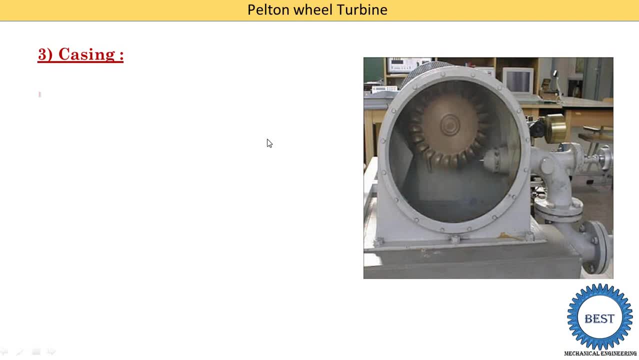 that is known as the casing. the casing is provided for a three different purpose. so first is to avoid the splashing of waters. when we run the turbine, the water is splash outside, so it's avoid the splashing of the turbine. second, it's avoid the accidents. and third one, it's guide the water in a tail. 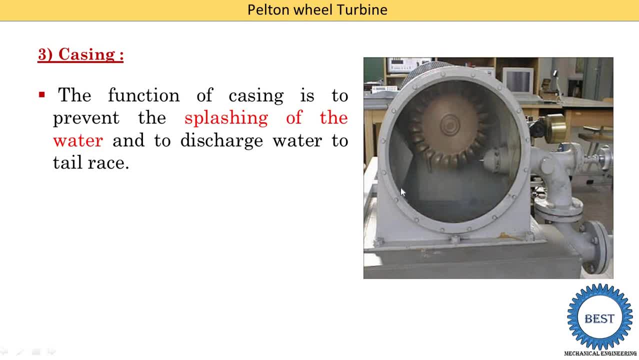 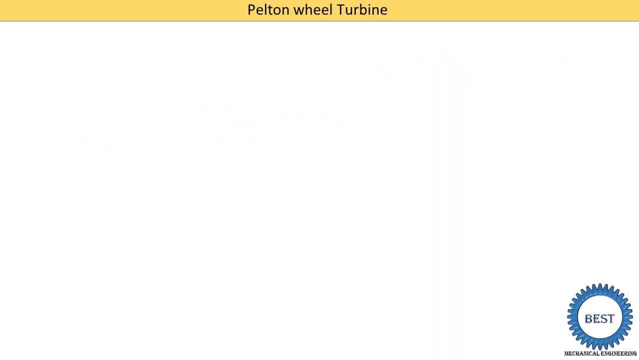 race means whatever the water is splash, it is a guided by the casing and the water is supplied into the tail race. so these are the main three purpose of the casing. and next and last component is the breaking jet. so breaking jet means why we are use the brake in our bike. so in a bike we are use. 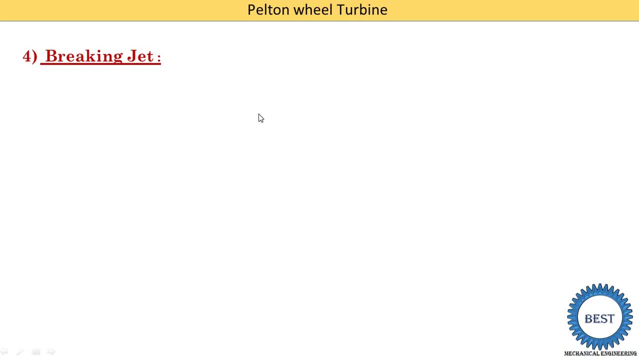 to brake, to stop the vehicles or reduce the speed. that is a two purpose. so similarly, this purpose is use in a pelton wheel turbine. so when the we require to suddenly stop the turbine, first we flowed close the flow rate from a nozzles, then after this turbine is rotated, 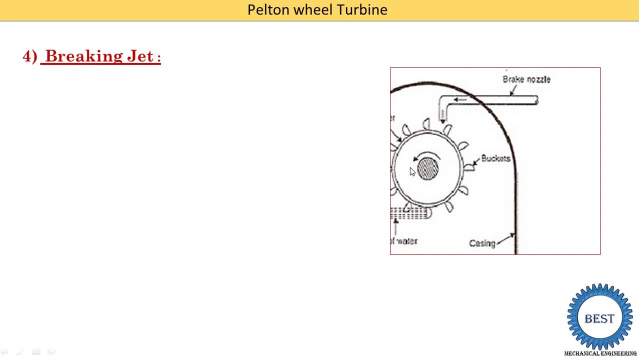 due to its inertia force. similarly, when we stop this engine of our bike, the bike is move on certain distance due to the inertia force, so that's why we are applying the brake to stop the bike immediately. similarly, similarly, when we close the nozzle valve, then after this, the runner is rotated due to inertia force and we require to stop the runner immediately. 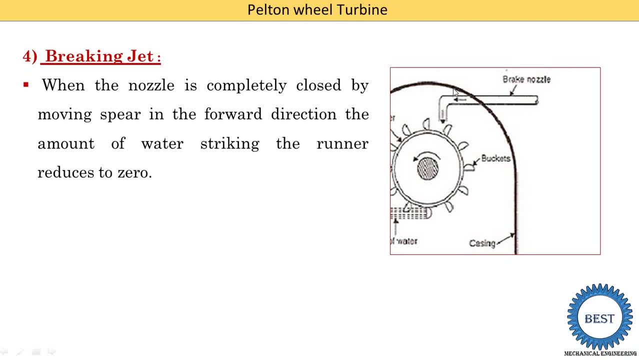 then what happen? we are supplying the some water quantity in the backward side of this bucket- ok means back side of this bucket- and we are try to stop the runner immediately. so this is the purpose of the breaking jet, similarly purpose of the brake in our bike. now the due to inertia goes revolving for a long time and stop the runners immediately. 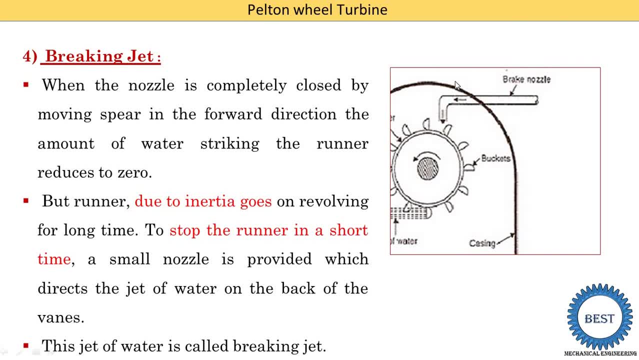 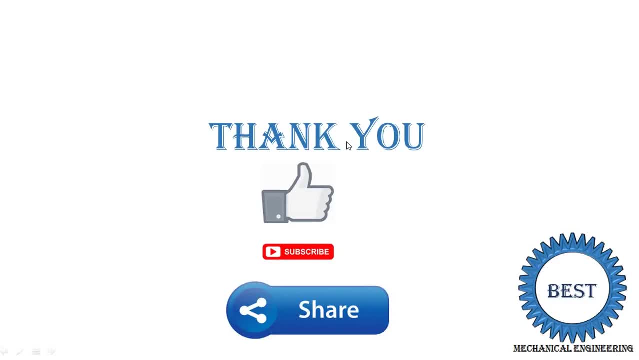 and this jet of the water is known as the breaking jet. breaking jet means it is used to stop the turbine runners immediately. thank you for watching this video. if you learn, then like my video, subscribe my channel, switch and share with your friends.